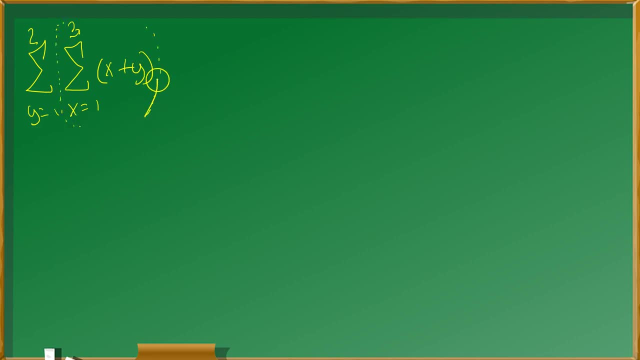 Group it in your mind as this: Let's do that part and then after that. So first, because the y part is on the outside, you're going to plug in the value of y equals 1, first into the expression, And then you're going to add up over the x's. 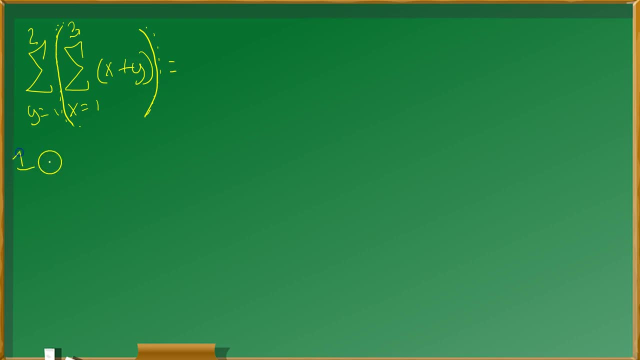 So, in other words, it's going to look like this: Take a look Down at step number 1, I will have this sum. Take a look. I'm breaking it into two individual pieces. x equals 1, up to 3.. 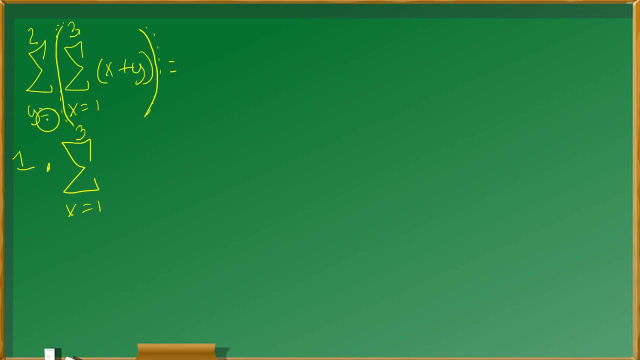 And the value of y will be first fixed at y equals 1.. So you put here, for that reason, x plus 1.. So this is the fixed value of 1 in this position from the outer sum symbol. And then you iterate over that, adding up. 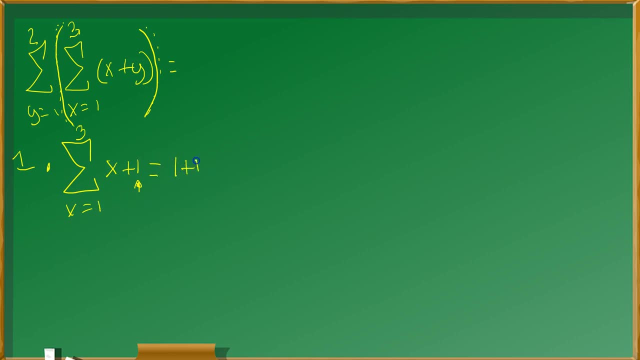 So in our case, that's going to give us the following: We're going to have 1 plus 1.. So here I'm plugging in. for each value of x, x goes from 1 up to 3.. So the next value of x will be 2, so it's going to be 2 plus 1.. 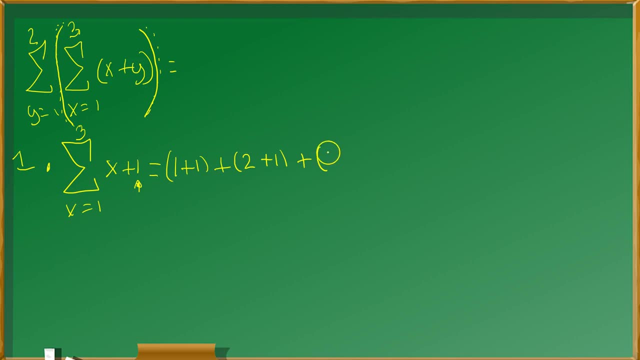 And after that I will have the last value of x, which is 3, so I will say it's 3 plus 1.. And notice, during this entire process you have fixed the value of y at 1.. And that's from the outer sum back there, okay. 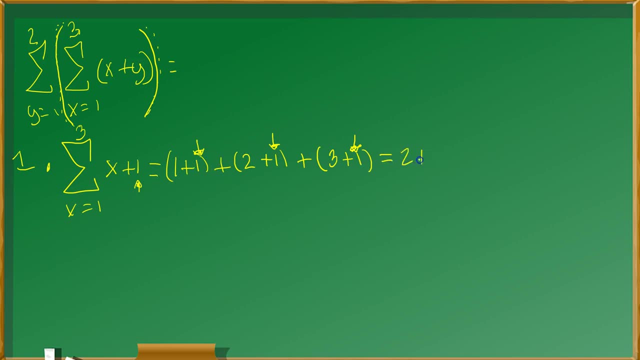 When I carry this out here, you will have 1 and 1, 2.. So it's 2 plus 3 plus 4, and that's a value of 9.. At the next stage in the process, you again go over the x's. 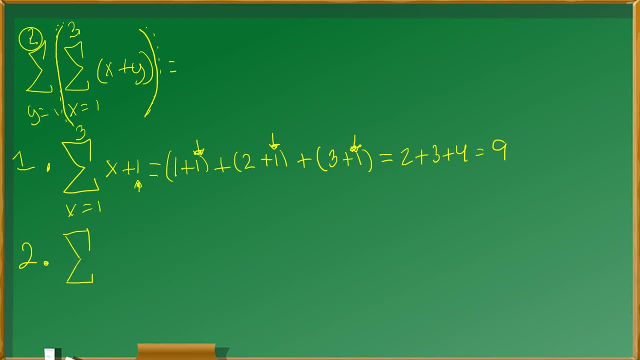 but you fix the value of y at 2.. So go back up to the top. You see y goes over from 1 on the bottom up to 2.. So for that reason here I'm going to put: x equals 1.. 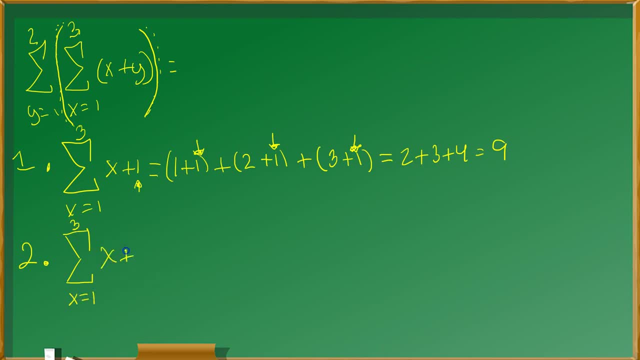 Up here I'm going to put 3.. And then, here for the expression, I'm going to put x plus 2.. And now this value, in this position, that 2, represents the stopping value of y- Go back to the double sum. 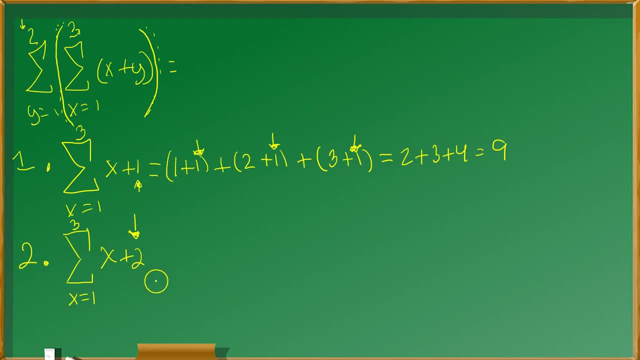 You see, up here it says that the y goes up to 2.. So I plugged in the value of 2.. I'm fixing the value of y, in other words, at 2.. And then I iterate over the x's. 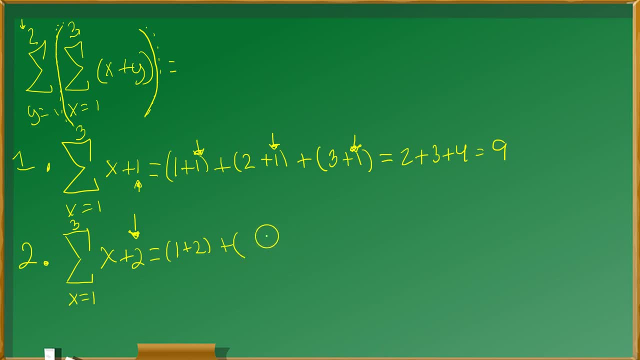 So when I do that, I will have 1 plus 2.. Plus here, I will have then 2 plus 2. And then, lastly, I will have here, let's see 3 plus 2.. You carry that out.